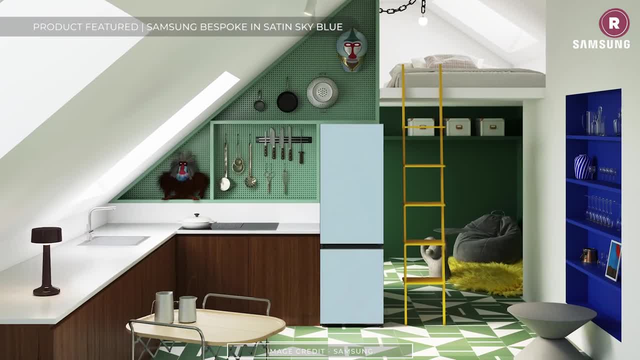 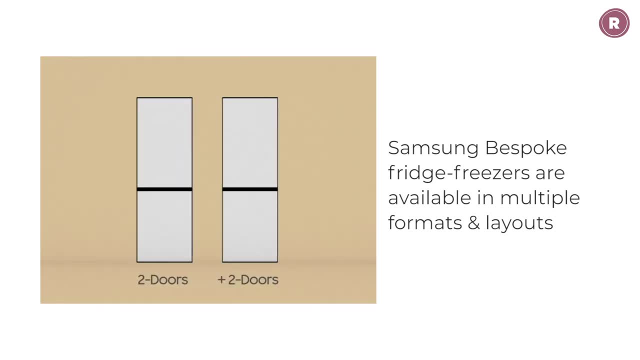 Not everyone has room for a giant American or French-style fridge with multiple doors, so look for something that makes the most of your available space. Samsung fridges with SpaceMax technology have thinner walls and this means more internal space without huge external dimensions. 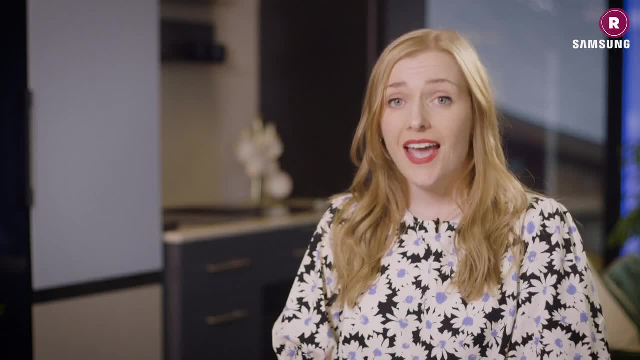 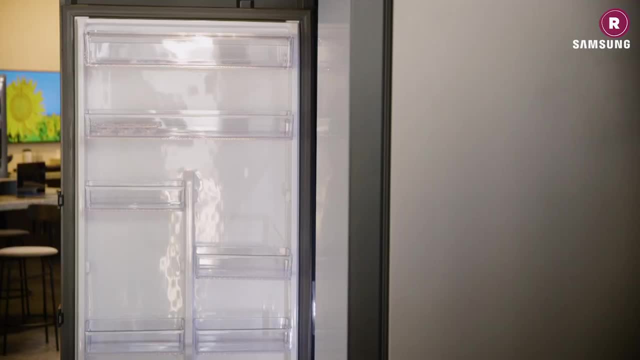 and there is no compromise on performance either. Next, think about the integrated storage features that can make a fridge freezer much easier to keep well stocked, yet tidy: Moveable door bins, slide-in or foldable shelves that can be moved to add headroom. 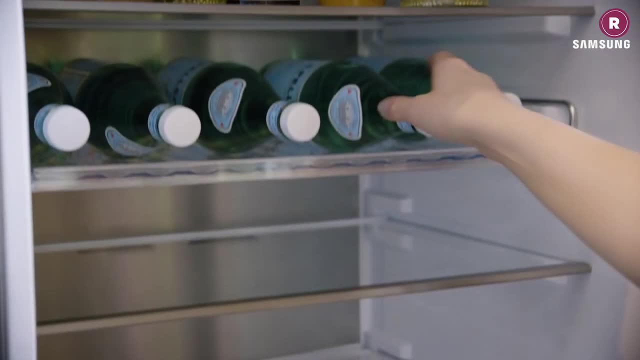 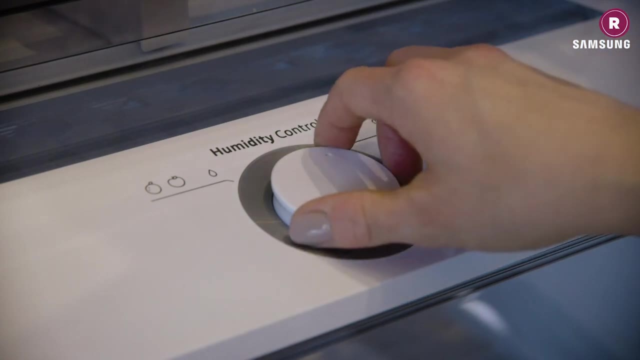 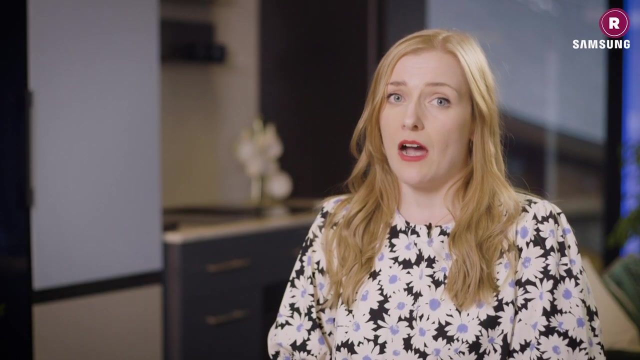 and, of course, a handy wine shelf, make putting shopping and leftovers away much easier. Generous vegetable crisper drawers keep produce neat and tidy while ensuring they keep food fresh, with humidity control, which is great when you buy too much. Keep an eye out for added temperature control too, like Samsung's Optimal Fresh Plus technology. 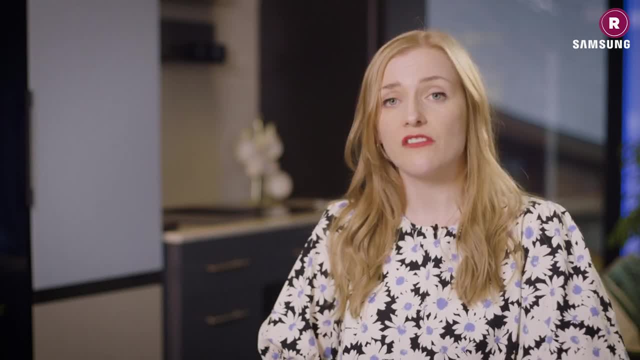 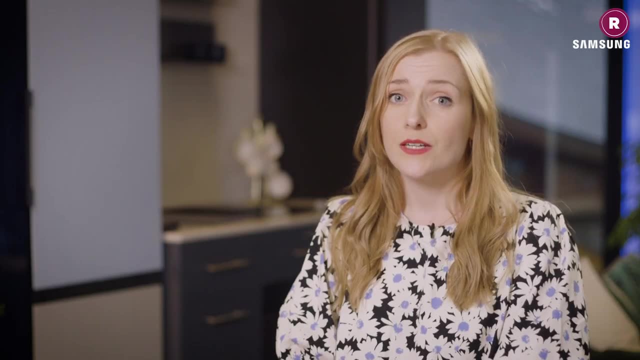 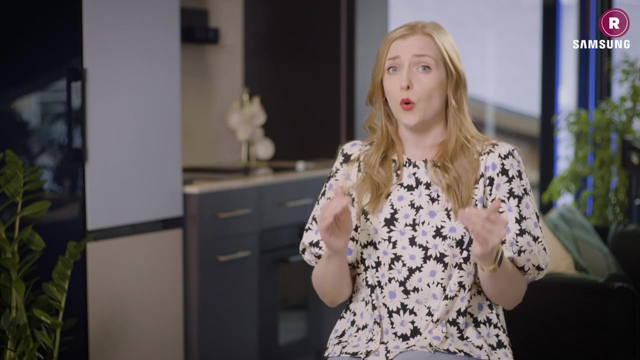 which lets you alter the temperature of the specific compartment within the fridge. You can make it cooler for meat and fish without chilling vegetables beyond their preferred temperature, which can impair flavour. Another function that helps you store your food at its best is choosing a fridge freezer that can rapidly cool or freeze produce when you return from the shops. 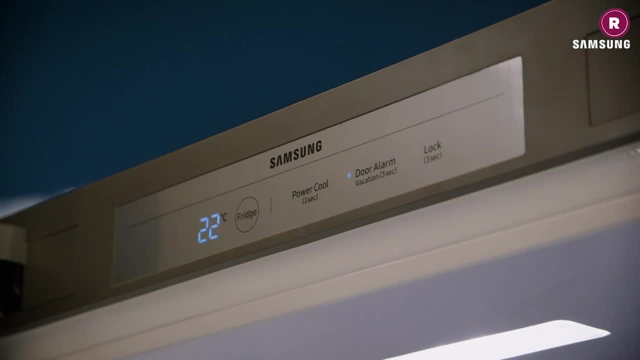 Samsung offers Power Cool and Power Freeze technology that quickly brings food back down to a temperature, a must if you spent a bit too long sorting your groceries. We also recommend choosing a frost-free option, as unwanted ice takes valuable inches from your fridge freezer space. 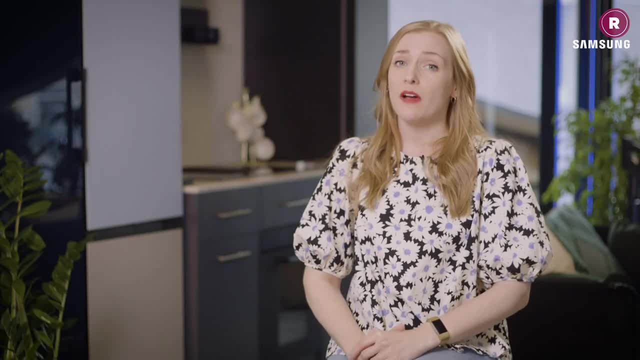 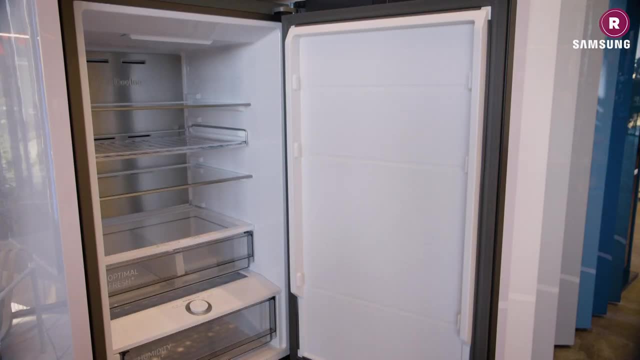 as well as being a pain to maintain. Finally, think about investing in additional storage that can help keep food not just fresh, but tidy in your fridge too. We recommend making the most of door racks, where they are available, for jars and cartons. 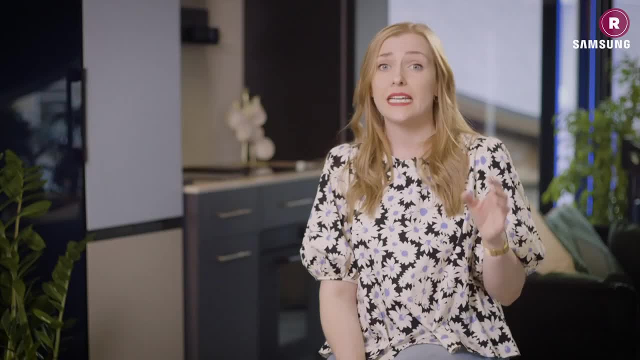 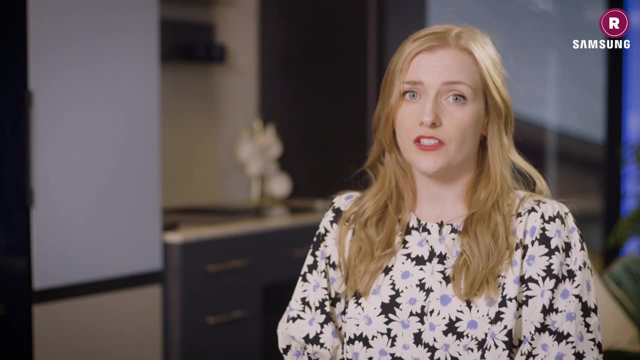 but when needs must, up your fridge storage game with clear bins to hold condiments or dairy products. This makes it easier to find what you need and remove contents to clean your fridge. A lazy Susan style turntable is another brilliant buy. no more underused items lurking at the back of the fridge here. 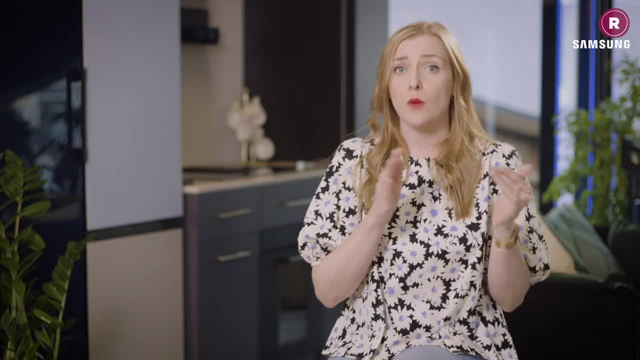 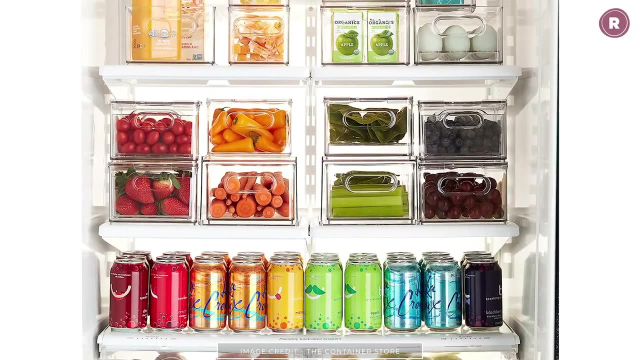 There are also some great food containers that can go from oven to table to freezer, both being used to cook and store your food. These are well suited to batch cooking and leftovers, and they limit the number of different items of ovenware you need. 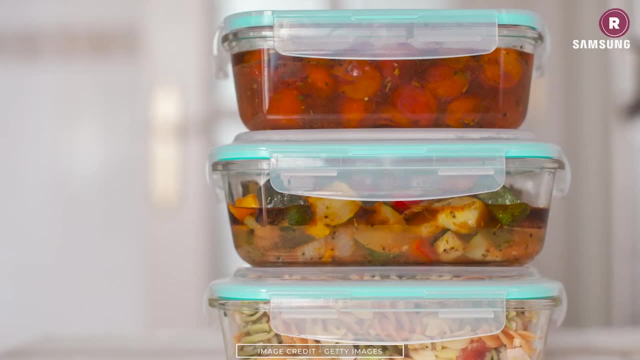 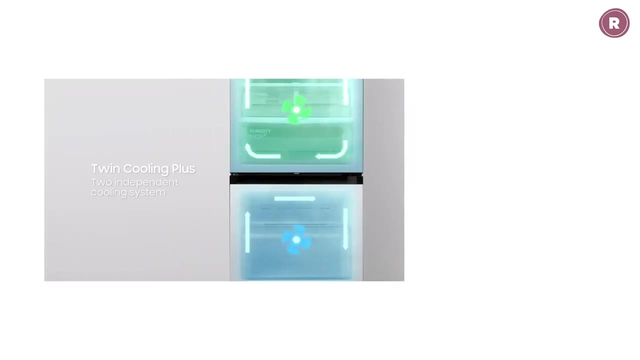 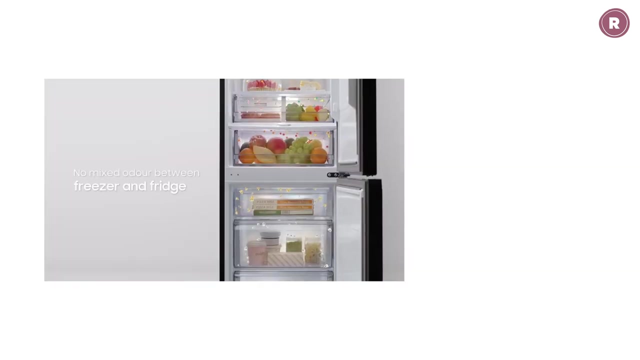 meaning tidier cupboards, too. Also, neat, airtight tubs will protect food in your fridge from taking on smells of anything pungent, though. Samsung Twin Cooling Plus technology is also designed to prevent odour mixing in your fridge freezer, making this less of a problem, so look for similar technology when you buy. 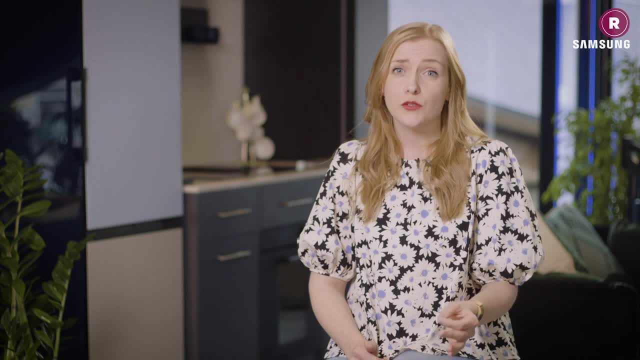 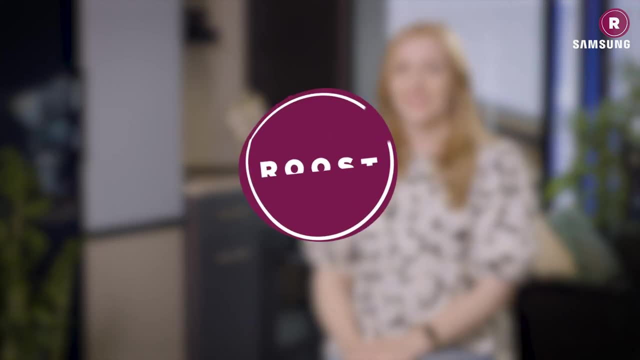 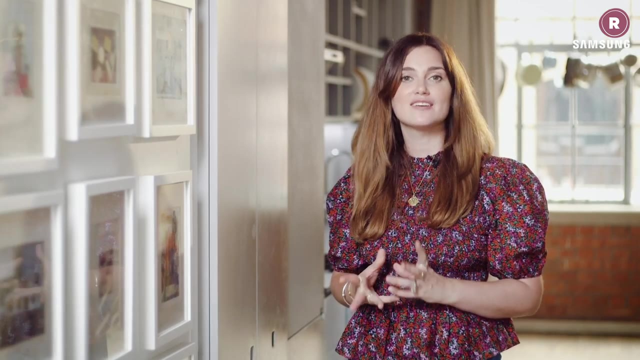 So there you have it. Just a few ways you can cut food waste while maximising storage space for a fridge freezer that the home edit would be proud of. If you want more ideas for fridge freezers, check out the Samsung Bespoke range. 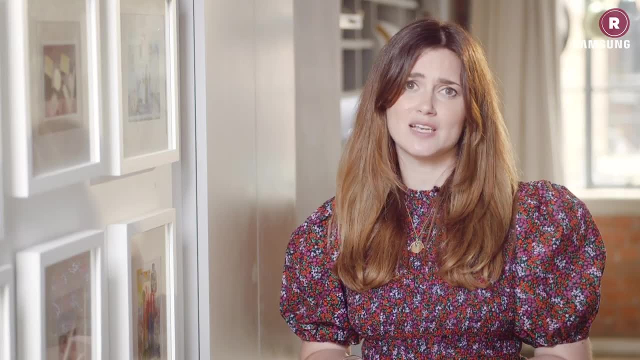 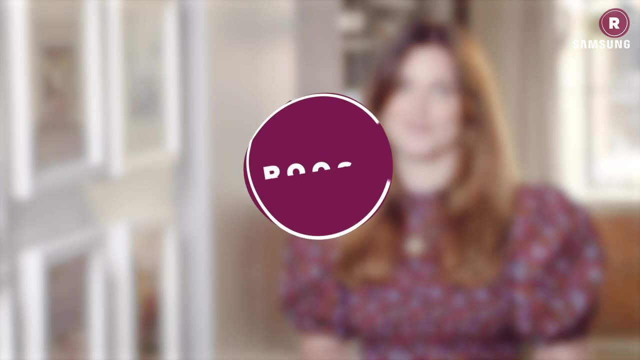 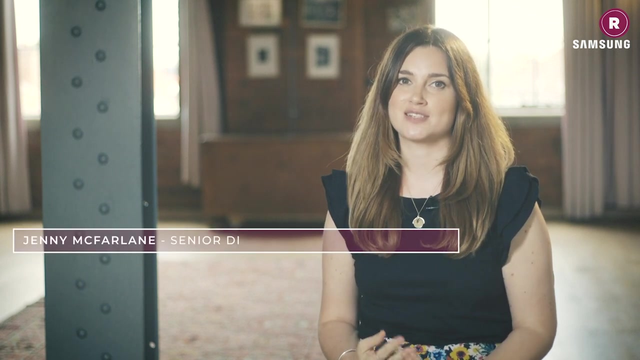 Now, if you want to ensure your bed is as comfy as it can be, I'm going to run you through my tips on choosing the best bed sheets. So you've got a good pillow, a supportive mattress or at least a mattress topper. 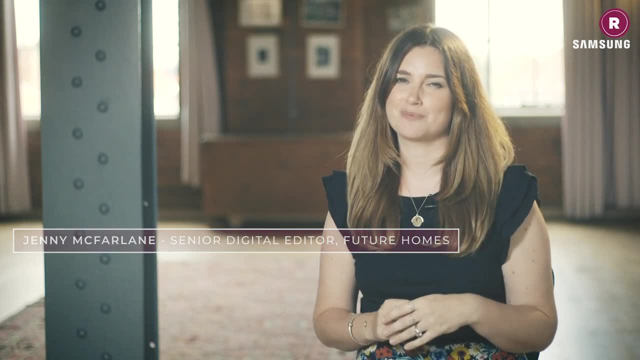 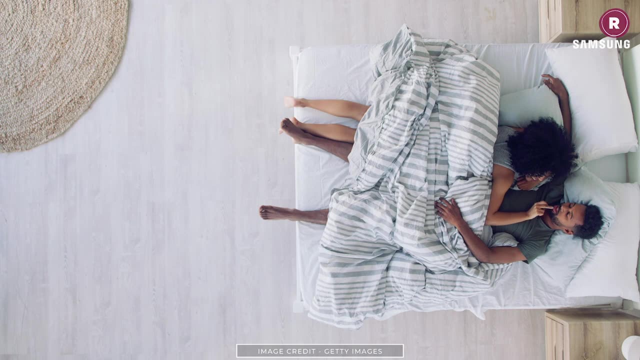 But if your bed sheets are scratchy, it's time to invest in some comfy sheets. We spend about a third of our lives in bed, and if you're struggling to get those much needed Zs right now, it's worth splashing the cash on some good quality bed linen. 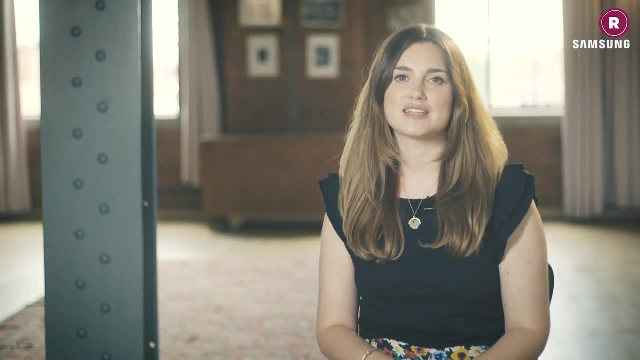 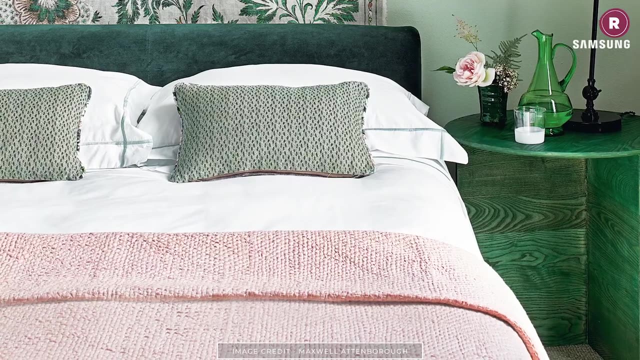 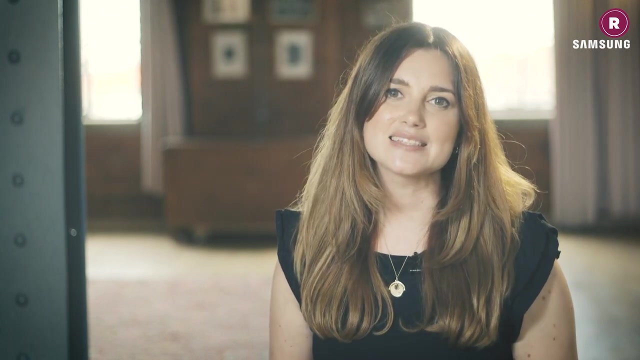 The most common fabrics for bed sheets are usually cotton, silk and linen, and luckily all of them are natural fibres which are breathable and help to regulate temperature. But they all have their unique characteristics and vary quite a bit in price. A classic, affordable bed sheet material is pure cotton. 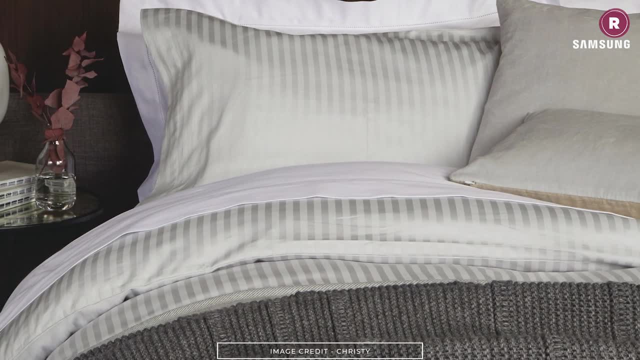 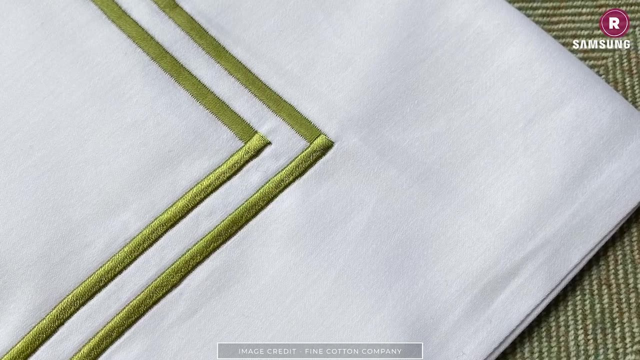 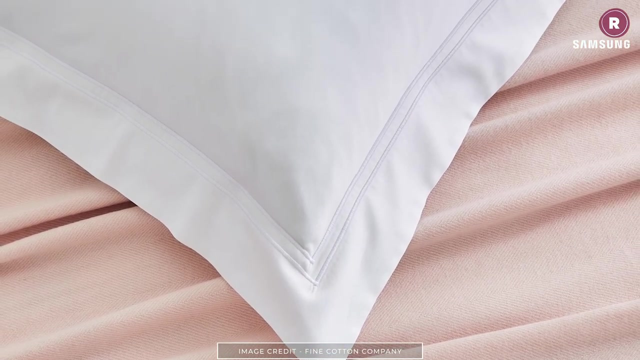 Egyptian cotton is one of the most luxurious types, with a smooth, crisp feel and a price tag to match. Egyptian cotton is longer lasting, finer and smoother than regular cotton, thanks to the extra long fibres that plants produce, which makes it a real worthwhile investment. 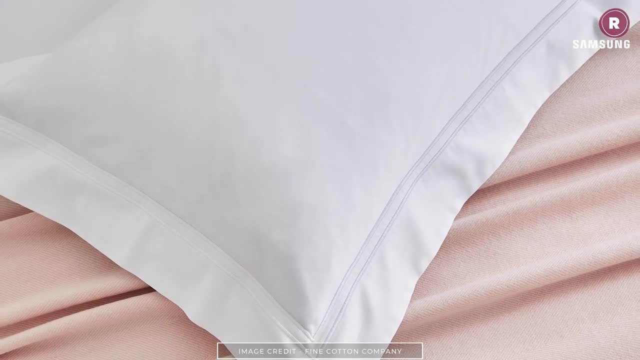 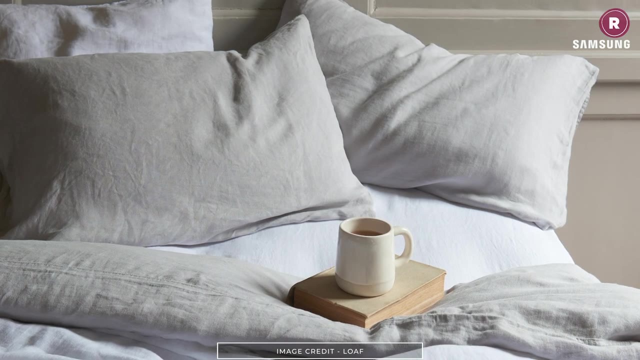 Be prepared to pay a little extra for linen and silk too. Linen gets softer over time, regulates temperature and doesn't retain moisture, so you'll be cool in the summer and warm in the winter. Just like linen, silk is temperature regulating too. 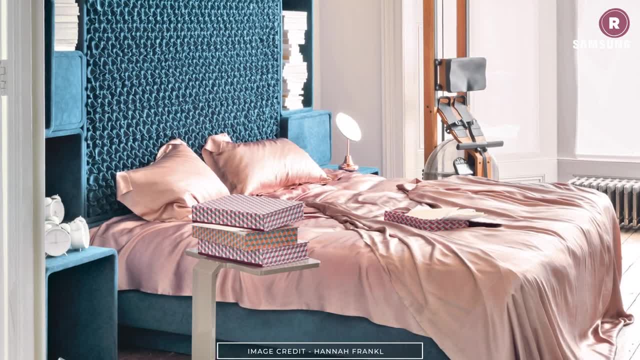 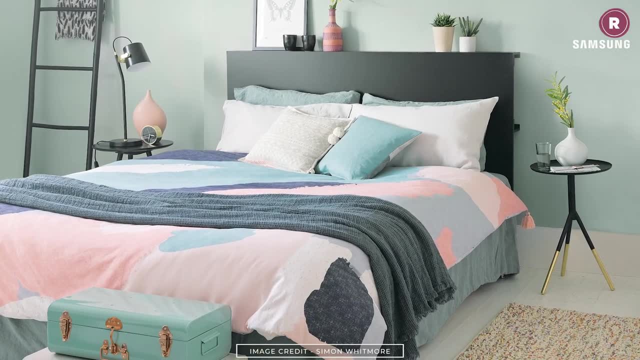 and also naturally hypoallergenic- perfect to help retain moisture in your skin and hair. You'll also find cotton polyester blends, which cost a lot less, are more durable and wrinkle resistant, but they may not feel just as natural or comfy. 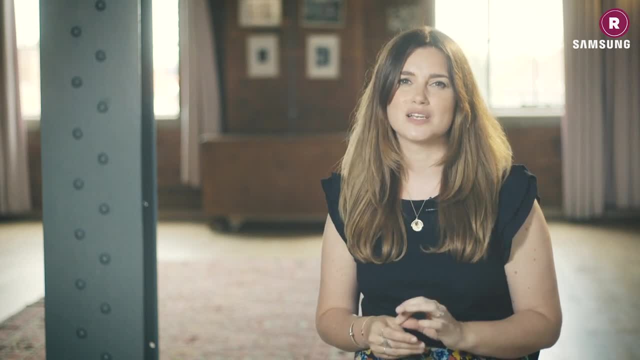 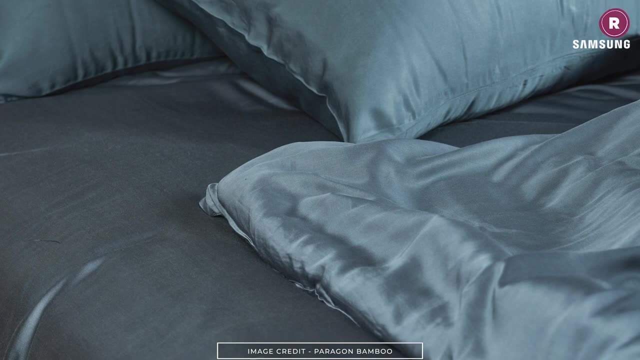 Your last choice is regenerated cellulose, also known as viscose or lyocell. These bed sheets are made using plants like bamboo and eucalyptus and are super soft, sometimes even softer than cotton, and often sustainably made. This one is linen. 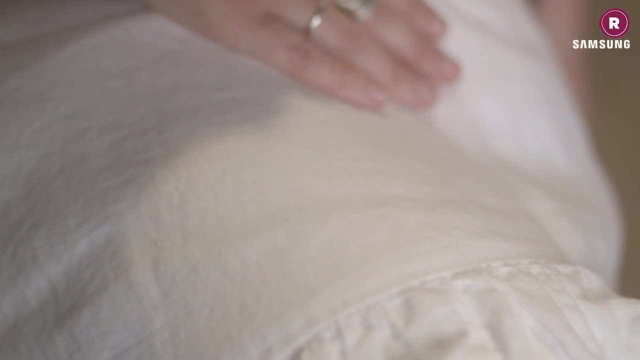 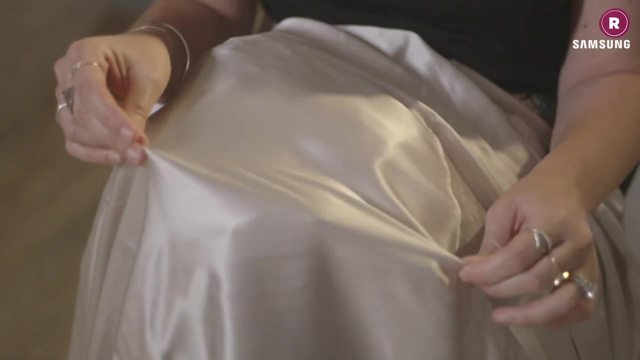 It feels sturdy, soft and crisp, while this silk sheet is much smoother, cool to the touch and has a subtle sheen. The way cotton sheets are woven has a big impact on how they feel. Your primary cotton go-tos are percal or sateen. 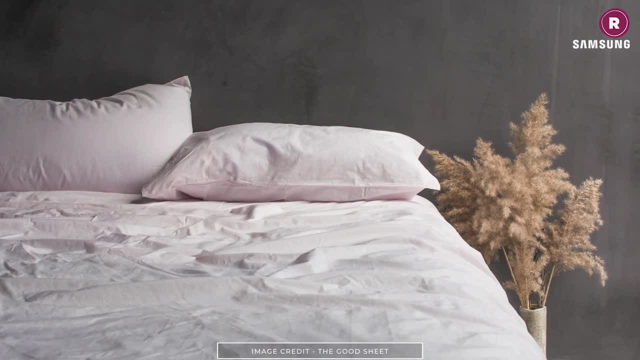 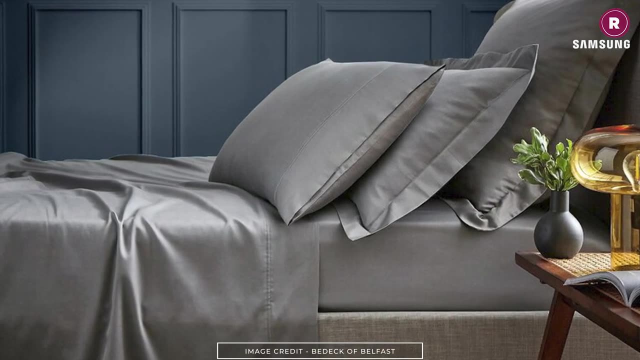 Percal is a basic grid-like weave and feels smooth and crisp and barely requires ironing, whereas sateen has a satin weave and is silky smooth and has a rather lovely subtle sheen. Jersey is a stretchy material which is less durable than cotton, sateen or percal. 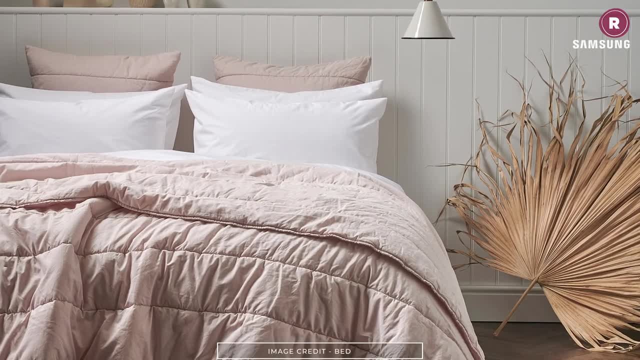 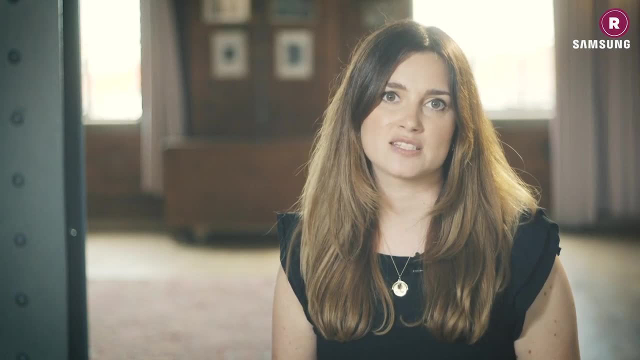 There's also microfibre, usually made from polyester or nylon, which is soft and fairly affordable, and flannel brushed bed sheets, often made from cotton or polyester, that feel warm and cosy in the winter. Referring to the total number of threads. 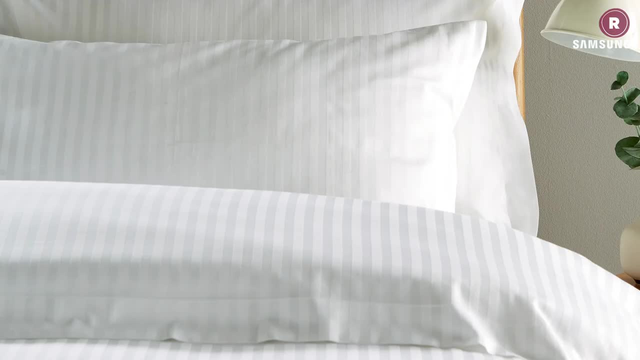 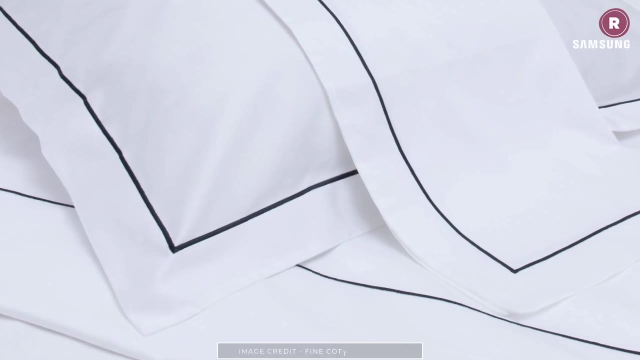 in one square inch of fabric. a high thread count is associated with a good quality cotton because it's known to make the sheet soft and more durable. A sweet spot of about 200 to 500 thread count sheet is all you'll need for a smooth, silky feeling. Fibres like linen or silk don't have thread counts comparable to cotton. As linen is so thick, the thread count is low, while silk is so thin that it's typically measured by weight, so you won't need to worry about the thread count of these options. 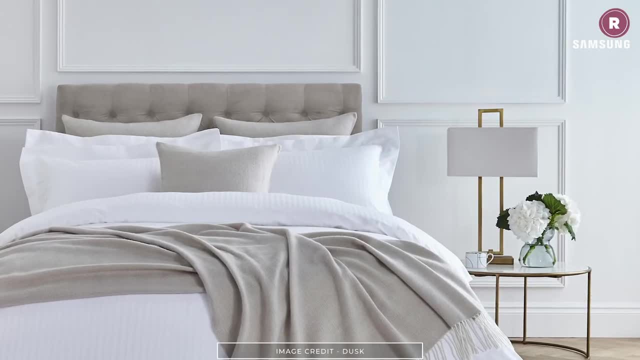 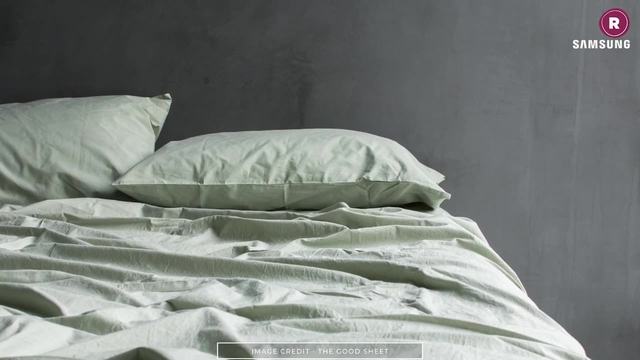 Whatever bed sheet type you go for, it's always worth shopping around for the best price and, if you can head to a homeware store to have a feel of the sheets for yourself, For more information and ideas for bed linen and textiles. 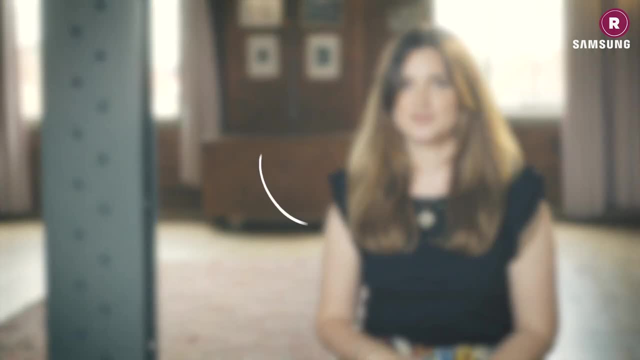 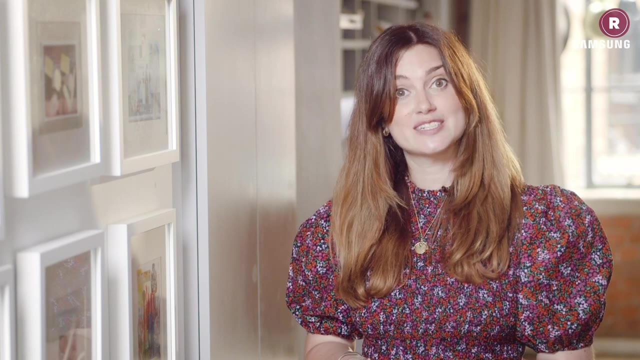 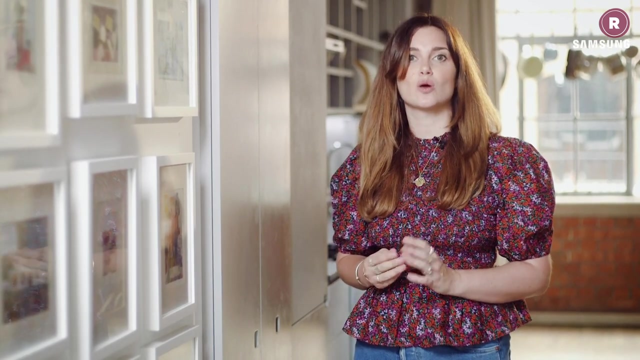 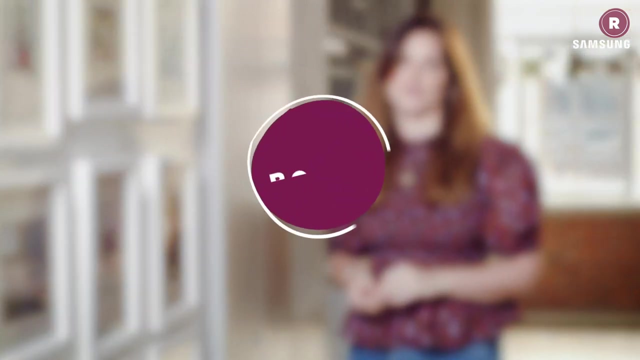 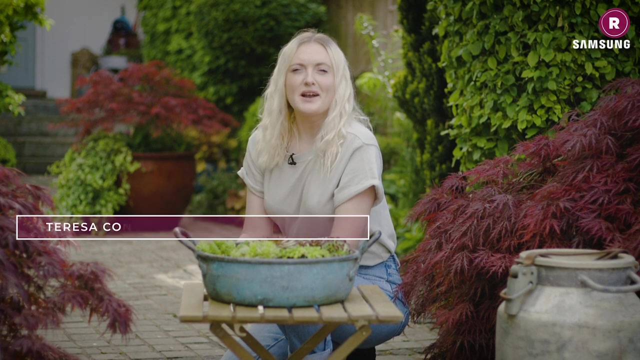 head to realhomescom, And now you know your sateen from your percal Next up. gardening expert, Theresa Conway shows us how to arrange a winning succulent scheme guaranteed to keep them alive and kicking. It's no wonder that succulents have taken the plant world by storm in recent years. 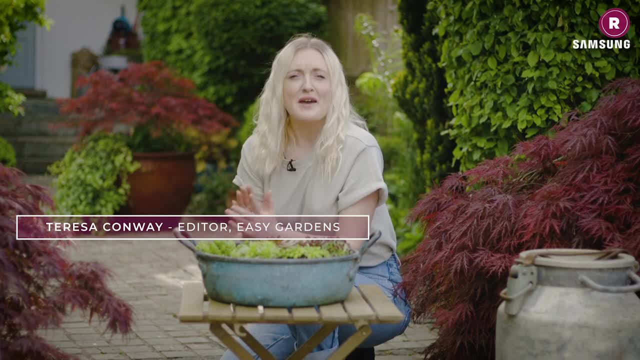 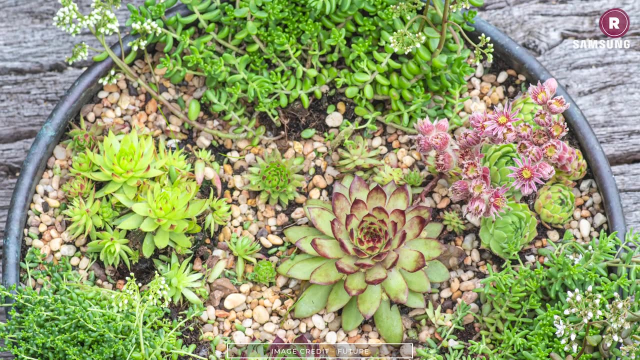 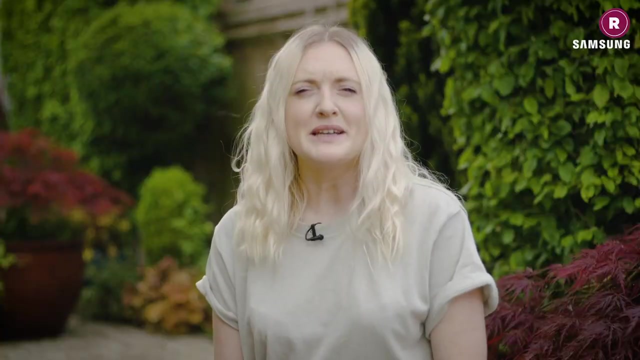 Aside from their beautiful structures and vast array of shades, they're surprisingly easy to grow. Some varieties will need to be brought inside during cold periods, but given that they make great houseplants, that's hardly a problem. Their popularity means that succulents are widely available. 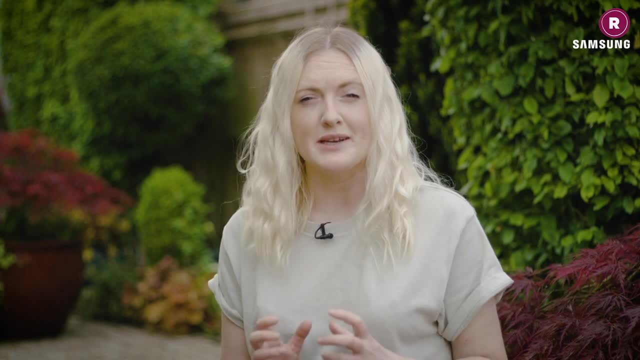 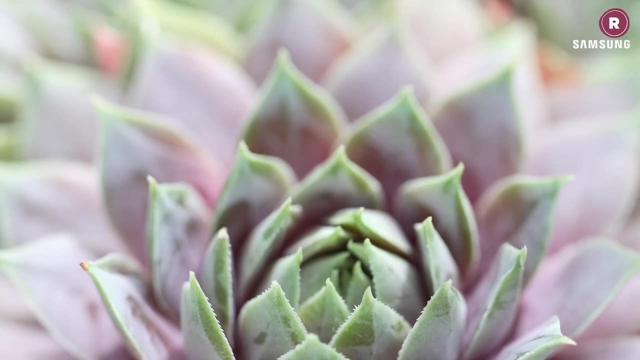 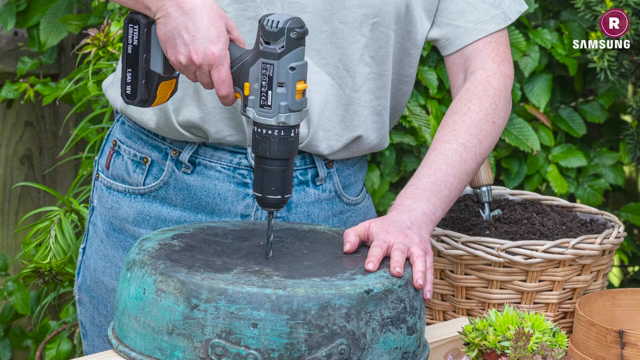 and you can really enjoy selecting your own combinations when planting up a container. They're so characterful and quirky that it really comes down to personal taste. Perhaps the most important thing to remember about succulents is that they require excellent drainage, so drainage holes are an absolute must. 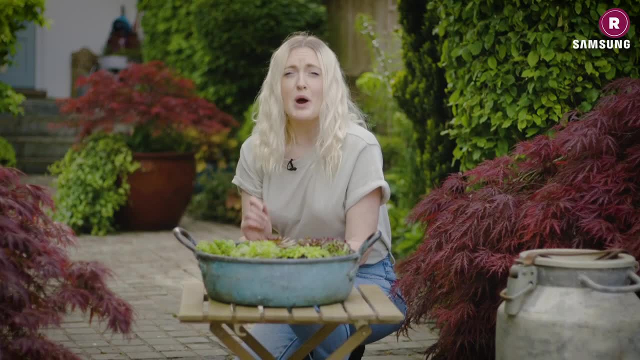 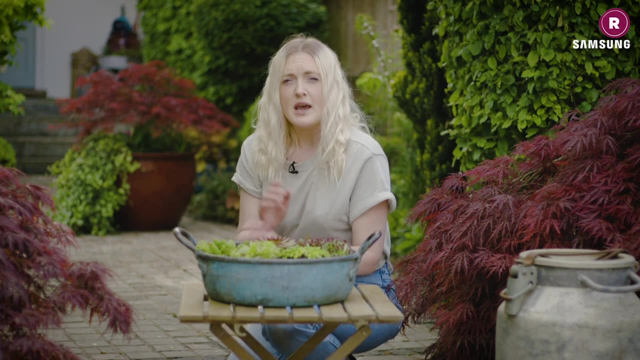 in whatever pot you're planting in. It is possible to buy potting compost which is specially formulated for cacti and succulents. If you're using a standard potting mix, add fine gravel or horticultural sand to really enhance its drainage properties. 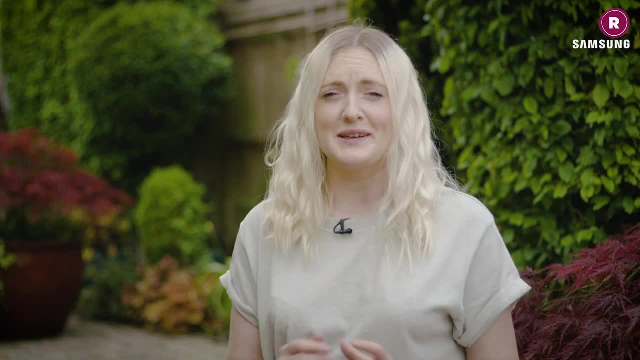 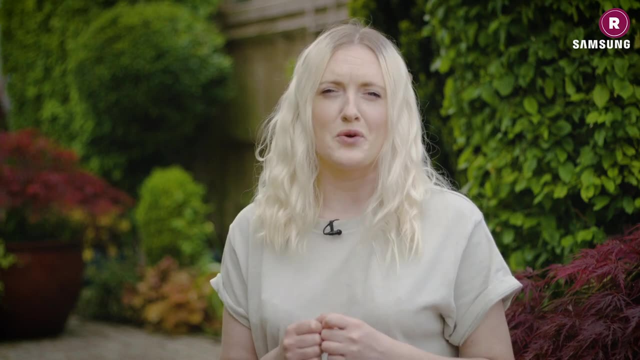 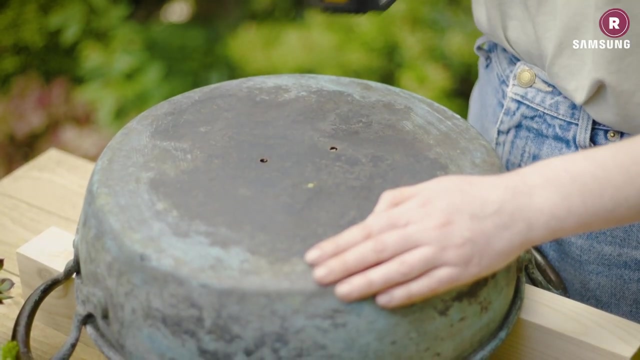 Here's how you can plant up a beautiful succulent container. We've chosen a shallow vessel with plenty of surface area to really show off the succulents in their full glory. As mentioned, your container needs to have good drainage, so we're adding some drainage holes to our copper planter. 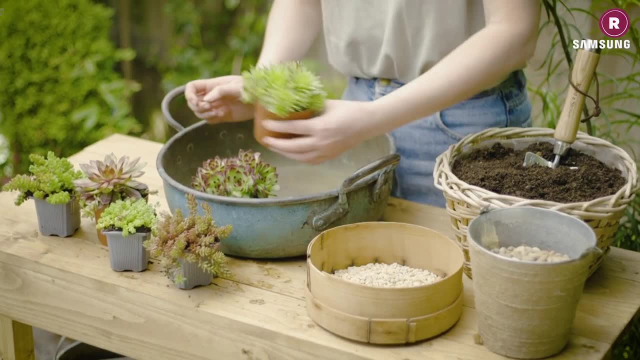 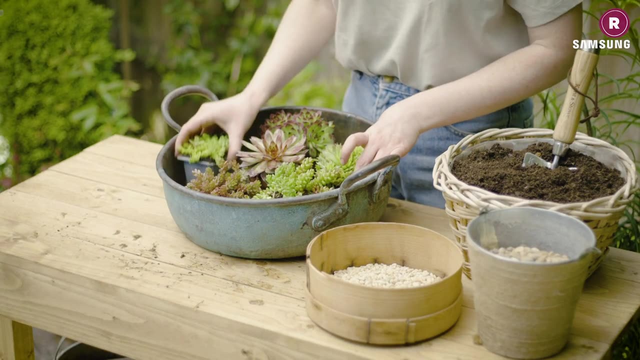 We've chosen a low wide bowl for our succulents, but it's an aesthetic choice and other types of well-draining pots would work just as well. To start with, we're arranging our chosen succulents in the bowl to check they fit. 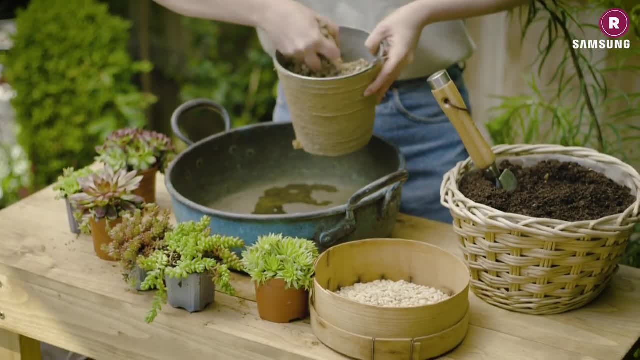 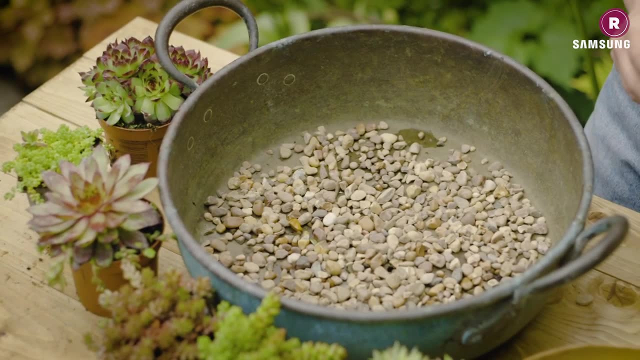 and look how we want them to look. Once you're happy, empty out the planter and add a good layer of gravel to the bottom to aid drainage. Succulents don't like waterlogged soil, so drainage is key. Now we're going to fill the pot. 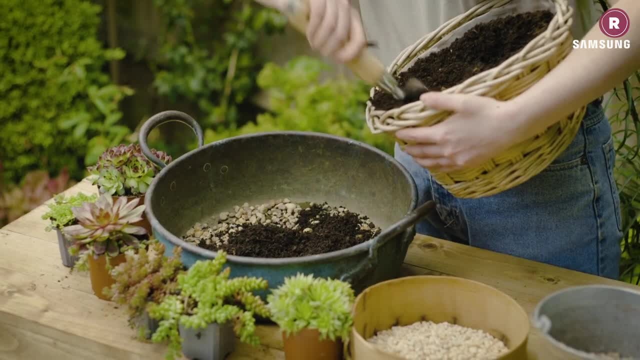 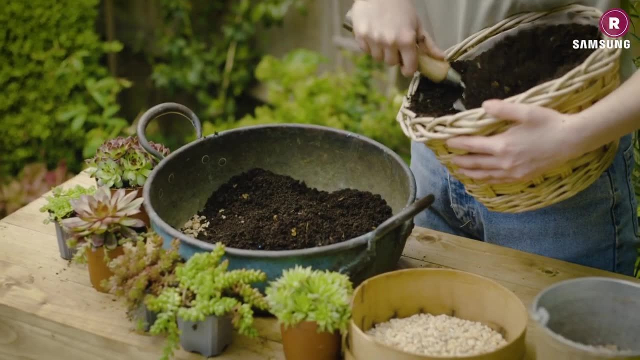 about two-thirds full with soil. The soil mix needed for succulents needs to be pre-prepared to ensure it has adequate drainage. We've done our own mix, which is 50% topsoil, 40% compost and 10% gravel. 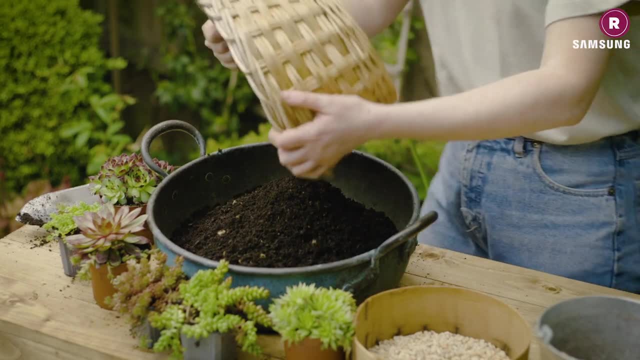 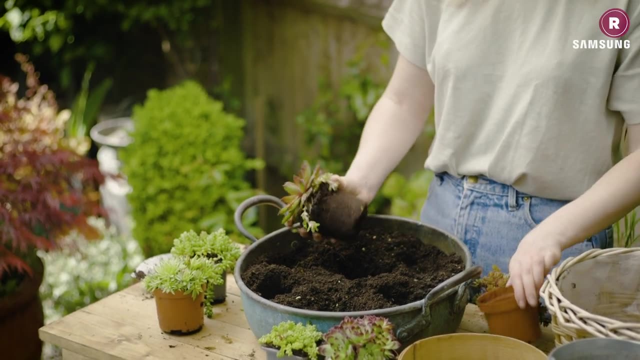 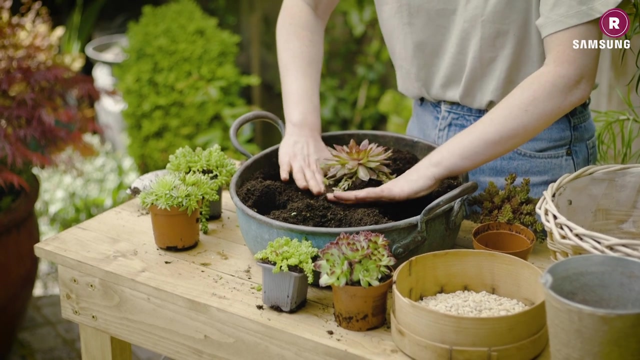 Or you can buy a ready-made mix from your garden centre which is specially formulated for succulents. Once the container is full of soil, you can start planting your succulents. We thought that the larger single Supervivum was ideally suited to sitting in the middle of our pot. 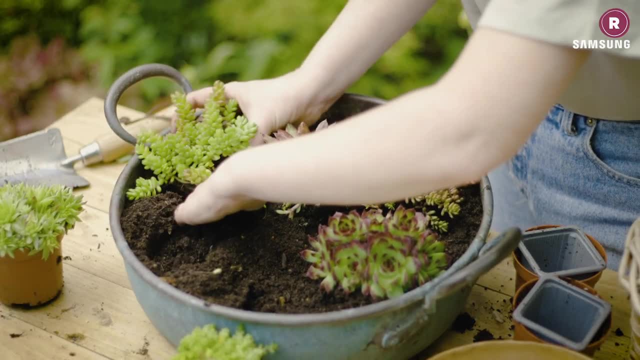 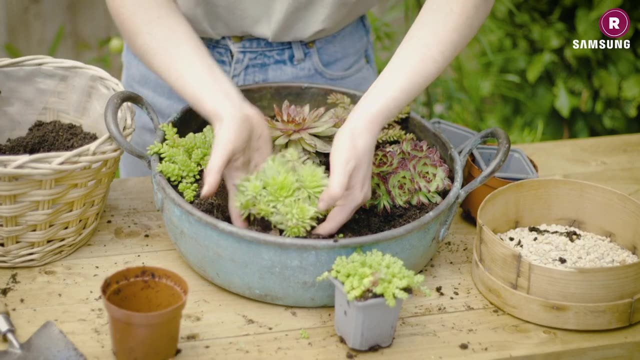 with the rest positioned around the central plant. But the choice is yours. Scoop holes in the soil slightly wider than the root ball of your plant and about the same depth, and gently drop the plants into place, firming the soil around them once they're in. 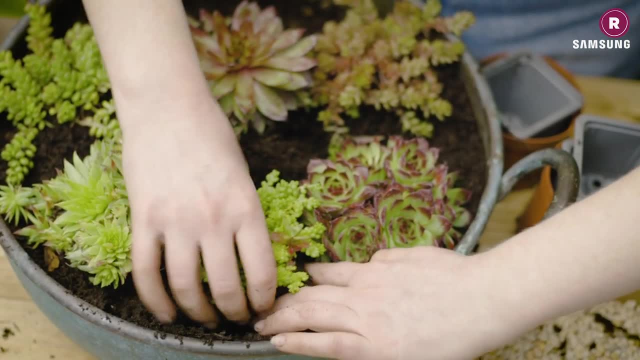 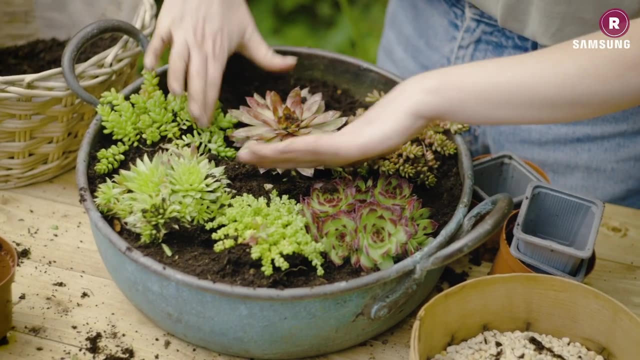 Once your plants are in, you can add a little more soil to level off the top of the earth and ensure that the plants are completely surrounded with soil. To top off the succulent planter, you'll need to cover the topsoil with horticultural gravel. 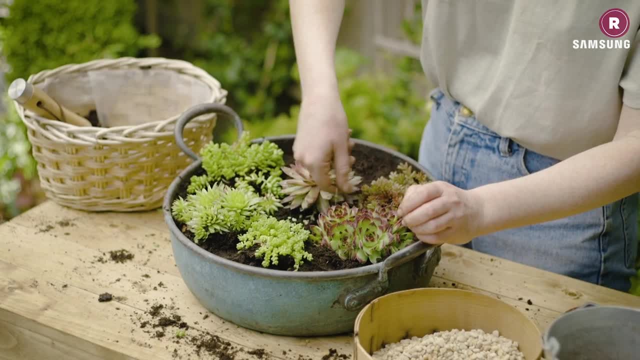 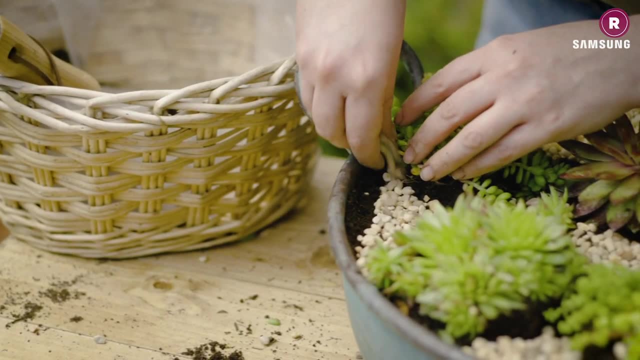 which stops the foliage touching the soil and rotting over time. It also gives a lovely overall look to the finished container. Ensure all of the soil is covered, including right up to the neck of the plants under the leaves. Finally, gently brush off any soil or dirt. 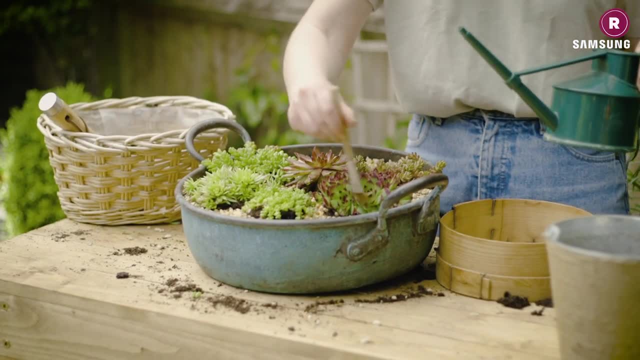 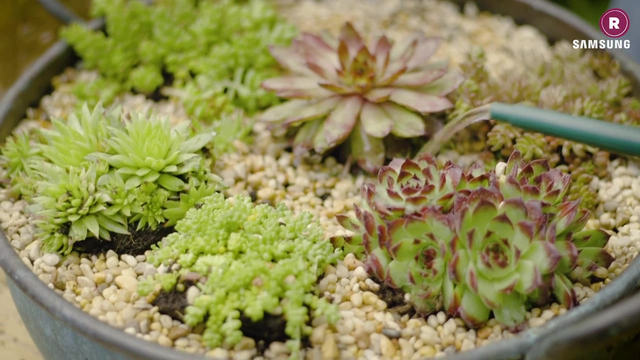 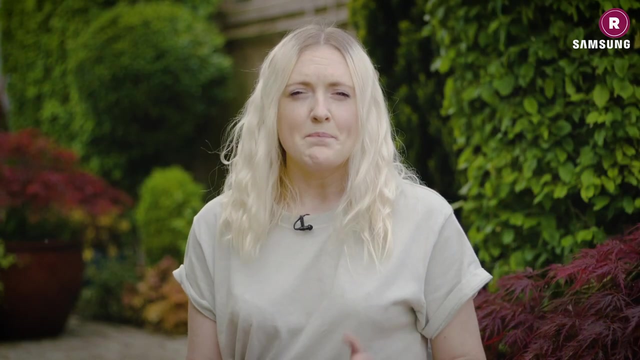 that's found its way onto the plants. Then finish by giving the plants a light water and position it in a partially sunny spot in your garden. Once you've finished your container, make sure you position it in a partly sunny spot When it comes to watering. 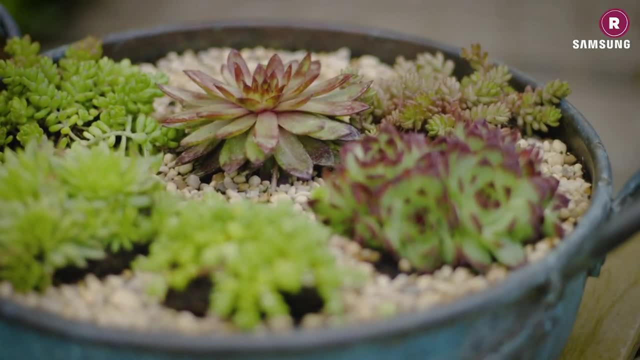 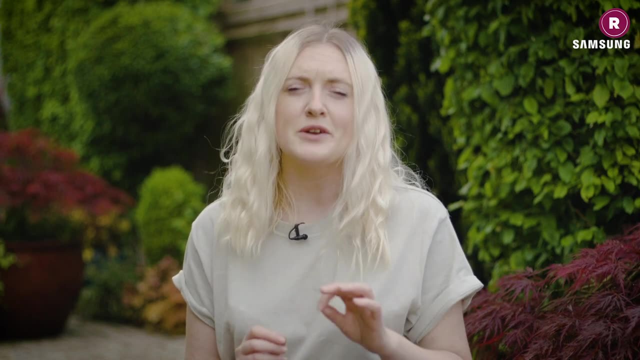 it's as easy to overwater as it is to underwater, And if the leaves come into contact with wet compost, they will rot, which is why we've recommended a layer of fine gravel on top of soil. Allow your container to dry out completely between waterings. 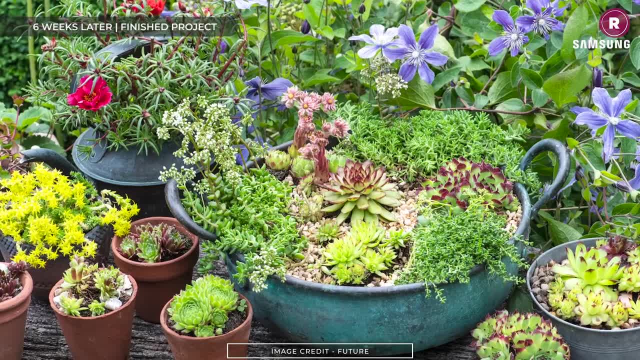 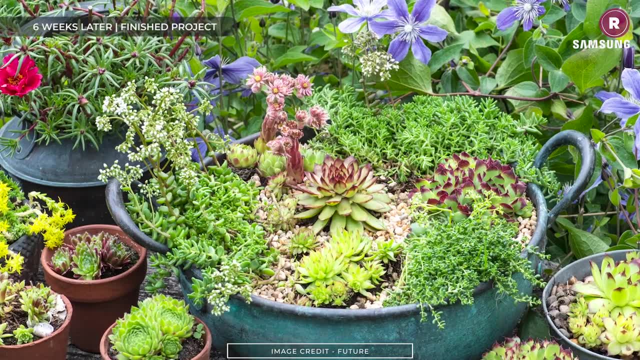 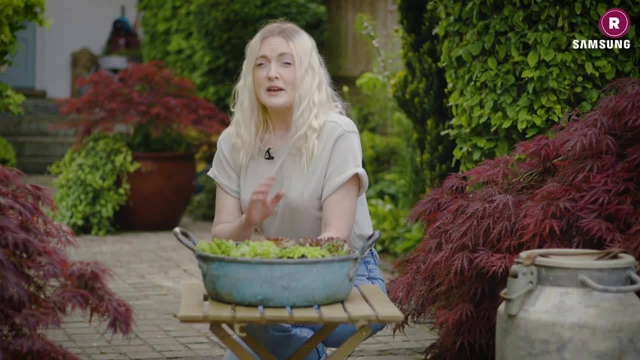 Check the soil regularly, as the period between watering will be shorter during hot weather. If the leaves are looking shrivelled, then they aren't getting enough water, whereas translucent leaves indicate overwatering. Remove dead foliage as it drops and, if you're using tender varieties,